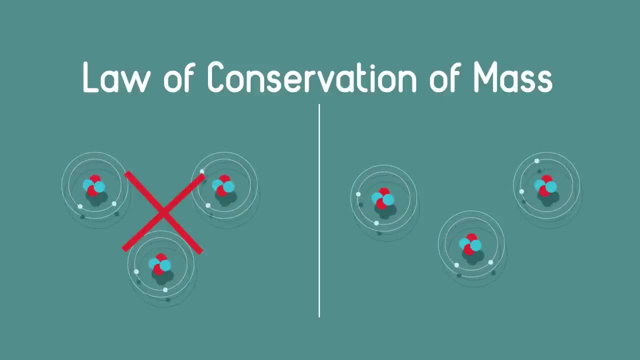 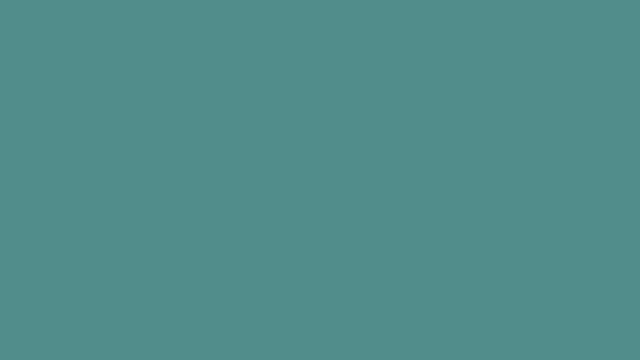 making an atom from nothing. The number of each kind of atom remains the same during a chemical reaction, even though they might arrange themselves differently in compounds. So here there are six oxygen atoms, And here And here, But these are three different ways. 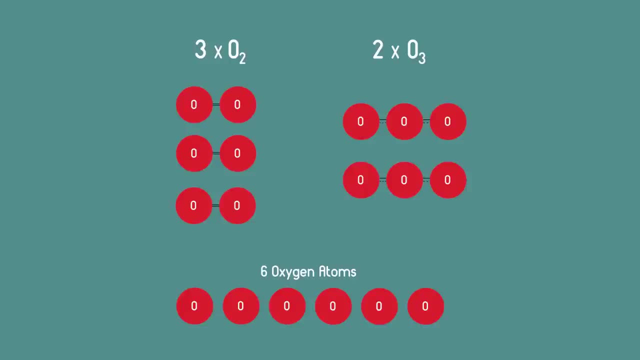 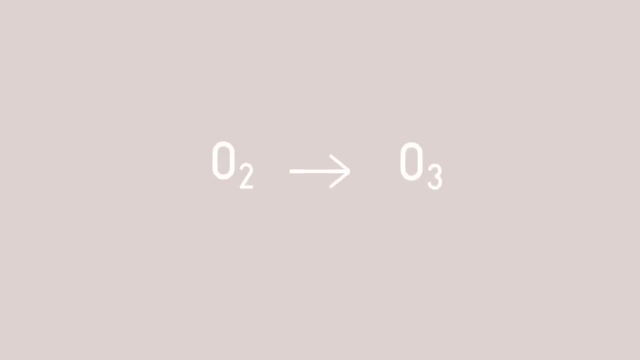 of arranging the atoms. Chemical reactions are all about rearranging atoms. Chemical reactions can be represented by simple equations so long as the number of atoms on each side of the equal sign remains the same. Often, when you write out chemical reactions, the 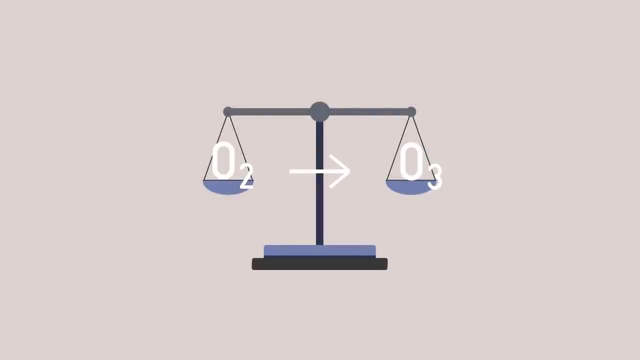 atoms do not balance straight away. You need to balance the equations to conserve atoms. You do this by putting numbers in front. Here we start off with 3 O2 moles In the formula. you can work out how many atoms there are by doing 3 times the subscript. 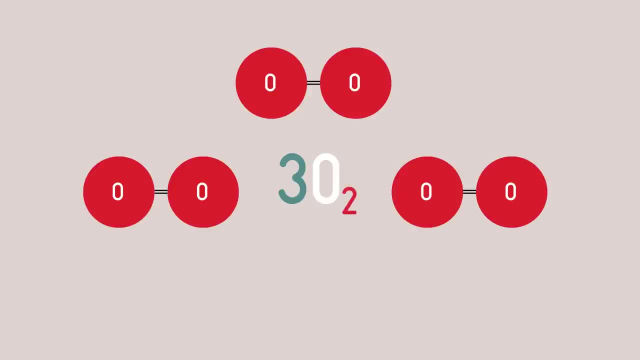 on the oxygen, which is 2.. 3 times 2 is 6.. Then we make 2 ozone molecules. The subscript is now 3, so the number at the front has to be 2, so that something times 3 is equal to 6.. 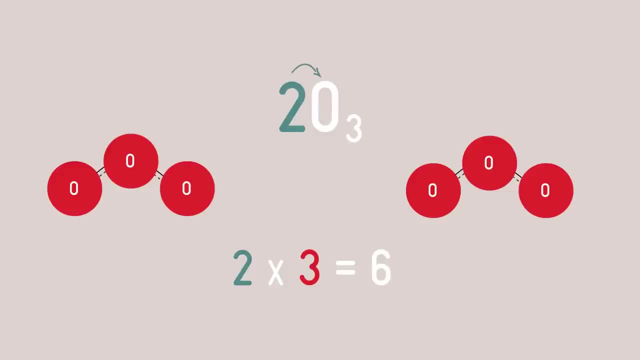 Here we start off with 3 O2 moles. Here we start off with 3 O2 moles. The big numbers at the front change everything in the formula, whereas the small subscript numbers only change the element they follow after. Until you are really familiar with using formula symbols like this, it's much easier to draw. 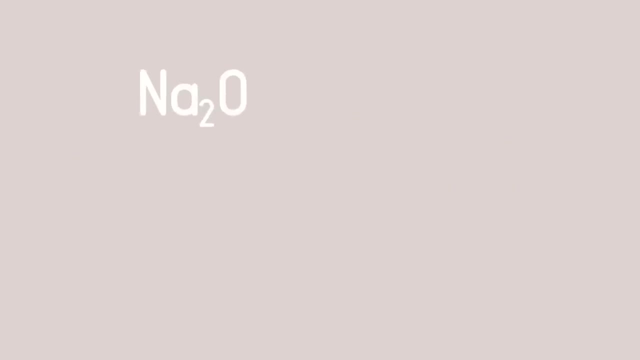